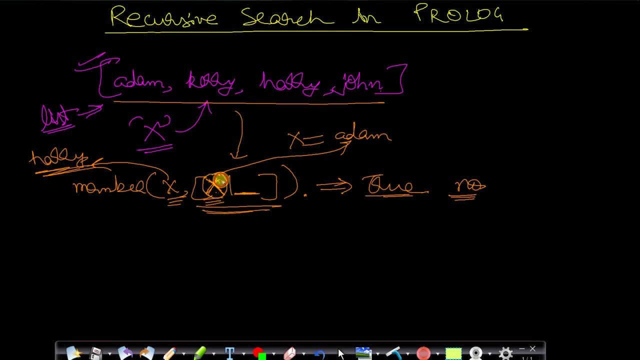 any other variable, you might ask why i have given here x as well as here x. this is given in order to denote that they both are same. okay, if they are not same, then the result will come out to be no. otherwise, it will come out to be true, no or false. okay, no or false. but if you want to give 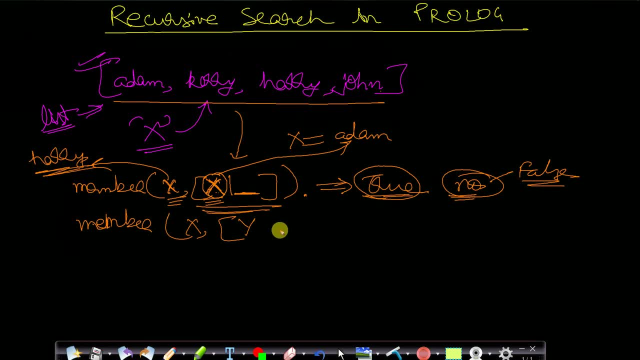 some other variable, then i will just show you how to do it. so, right here, member x, comma, let us save, give it y, then the anonymous variable and close it. and you cannot just give the full stop here. you will have to mention x is equals to y. so what this will do is this will return a true result. 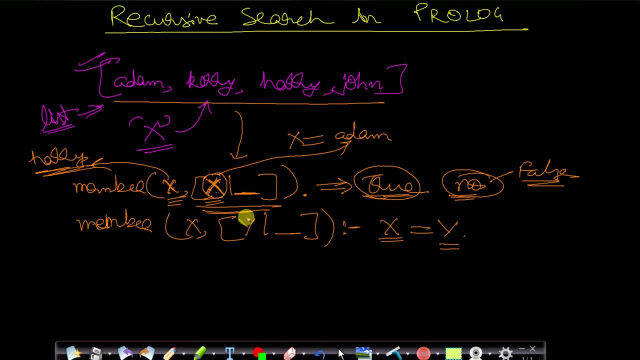 if x is equals to y, while when we had given x here or in place of this y, then it was implicitly done. that means the comparison between these two variables was implicitly done. okay, so there was no need of doing it. okay, so let us write the entire code. this is our first line. okay, and let 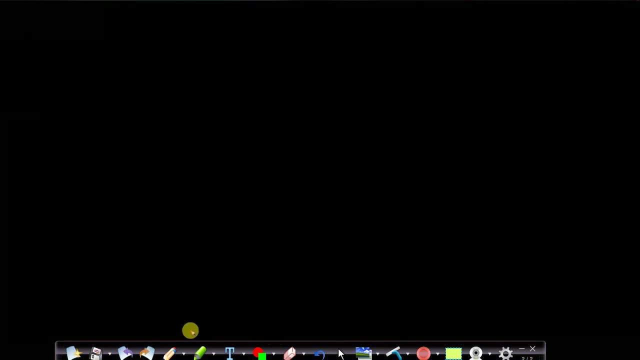 me clear it out and then we will write the entire code. so our list was adam, carrie, harry and john. okay, so this was our entire list. and let us say we want to search for the element x, which is harry. so how will the code work? the first line will be a fact: member x, comma x. okay, so what this will do. 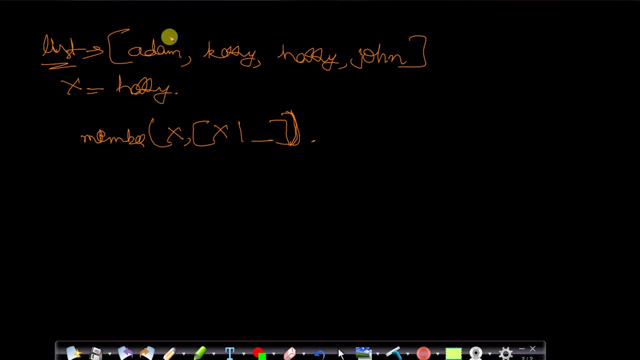 is that this will compare the element, the head of the list, this adam, with this harry, okay, and then we'll search whether they are equal or not. if it is not equal, then it will move on to the second line of the first line. and what is our second line? the second line of code should be a recursive one, okay. 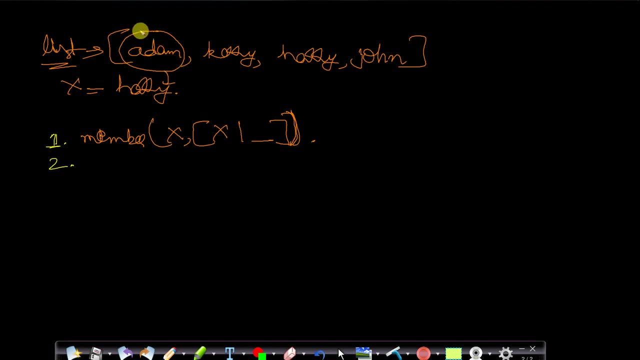 and what will this recursion do is? this will eliminate this first element and should look for the rest of the element. so let me just write the code in order to clear it out: member x comma anonymous variable. then give here y and then write member x comma y. so what does this mean? this means that x belongs to this list if x is a member of this list. 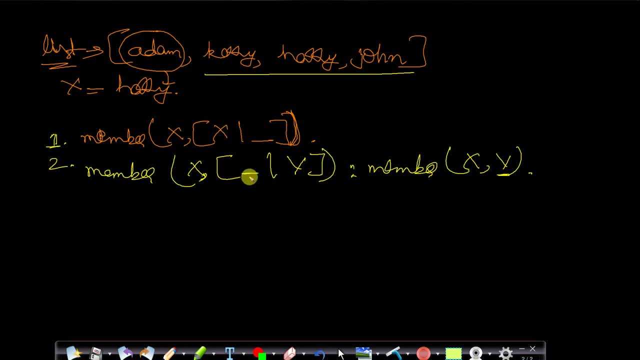 okay, so how is the list divided now? you can see that this anonymous variable now is assigned to the head part, so this anonymous variable will be equal to adam. okay, and what will this y be? this y will have three elements: carrie, harry and john. okay, 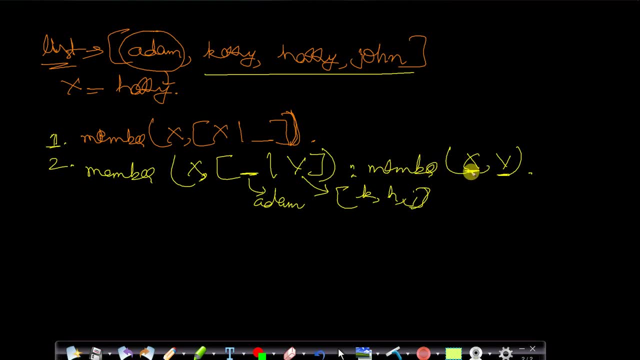 so now, what will be done is this: x will now be compared with the y. that means the rest of the elements, the rest three elements. so what? so where will the control go now? the control will again jump back to the first line. it is a recursive statement. okay, so again. member will be called. 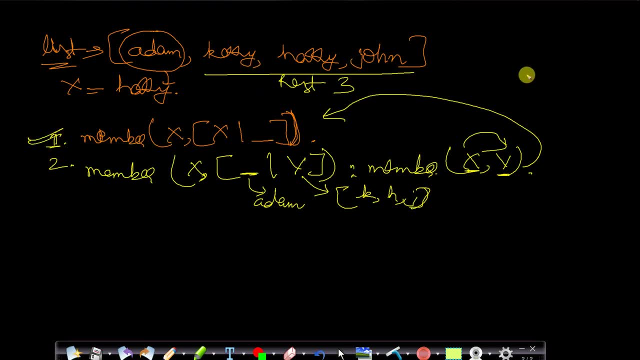 this line will again be called and here again, this list will contain only carrie, harry and john. okay, since this list has only three elements now, x will be compared against x, that means harry will be compared against carrie and they are not equal. then again this second line. 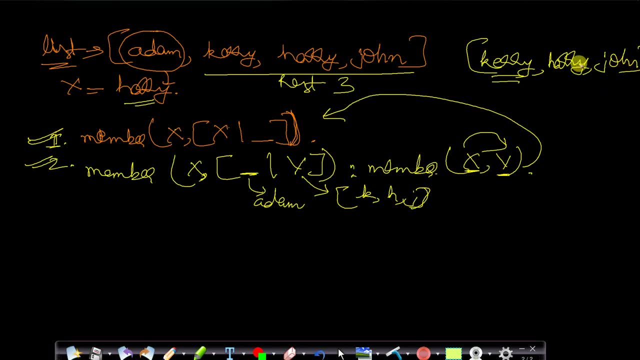 will run, and here the entire list will again be divided into two parts. this anonymous variable will now be equals to carry, and this list will now contain only two elements: harry and john. okay, and now this member? x means this person. x will be a member of the list. that means the member of the group if x is a member. 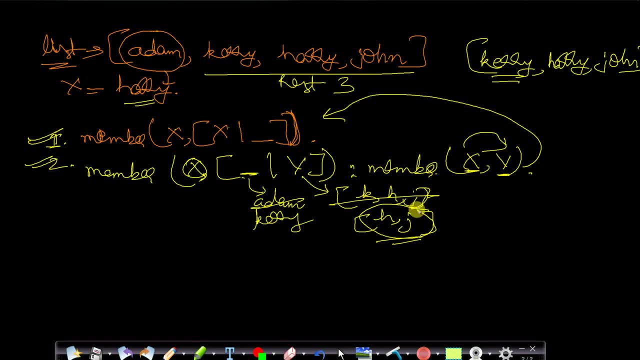 of y, that means if x is present in our rest of the elements. okay, so again, the recursive call will be made and the control will go back to line one. and again harry will be compared with the head of the list, and now our list has reduced only two elements: harry and john. okay, and now what will be done is: 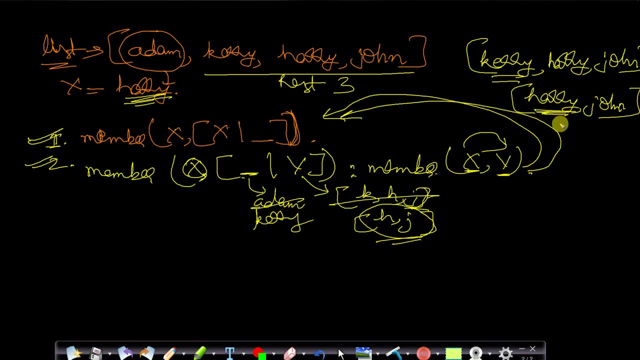 harry will be compared against the head of the list, which is harry, and so it will return true and our execution will stop. okay, so this is how we can write a recursive search code in prologue. so let us demonstrate the code using sweep prologue. 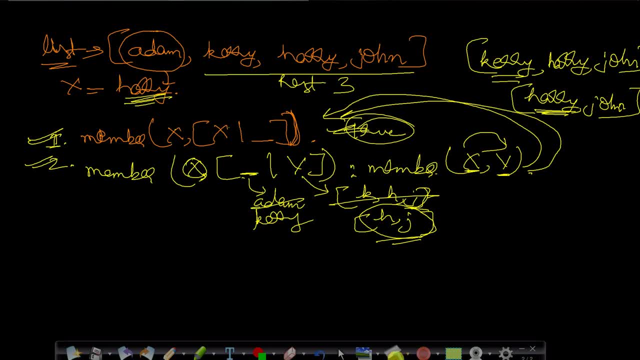 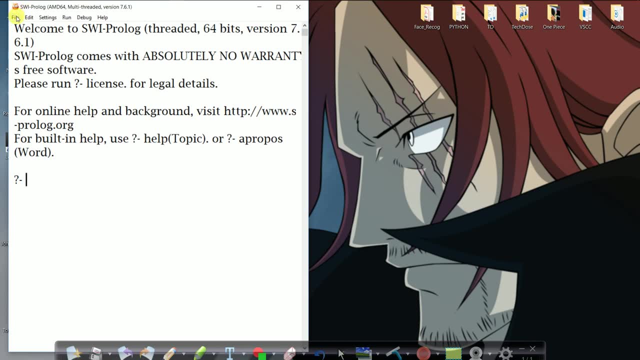 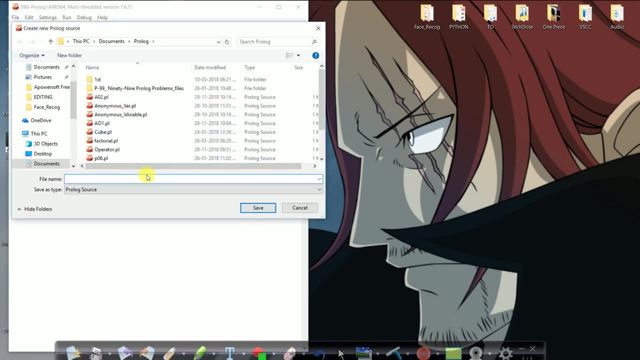 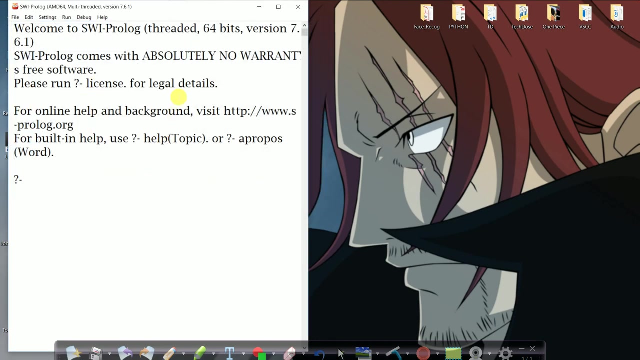 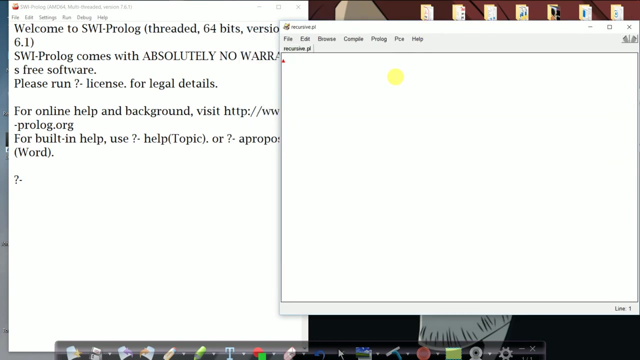 so i will just open sweep prologue. let me just change the control, okay, and now let me make a new file. so i will go here, we'll make a new file and let me just call it recursive dot pl. okay, and now my coding window will open, as you can see, and here i can write out the code as member. 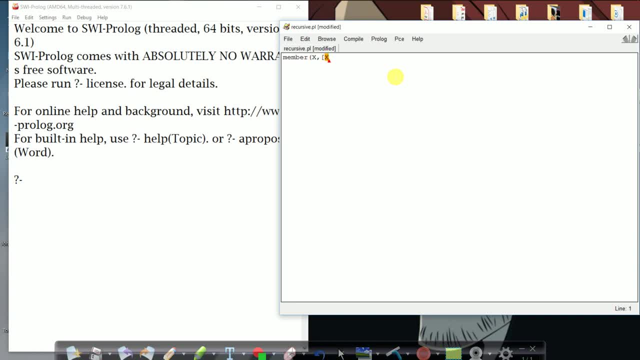 x comma x variable, the underscore, and then this is our fact, which has been declared, and then again we will write the rule, the recursive function call, and this will be y. you can see that we are repeating the same thing. member x comma y. so if you read this in english term, then you will be able to. 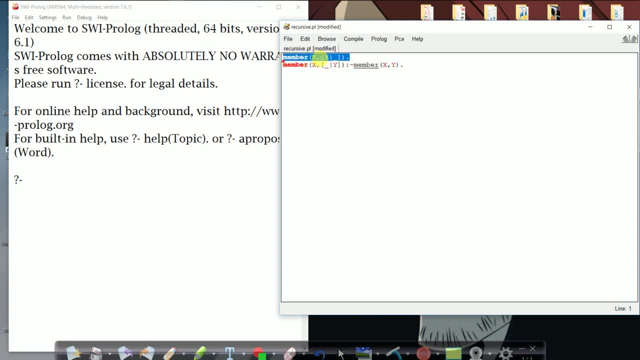 understand it very well. the first line indicates that x is a member of the group. that means the list. if the head of the list is equals to the elements which we are searching, then it will return true. otherwise, if this is not true, then it will move to the second line and it will search. 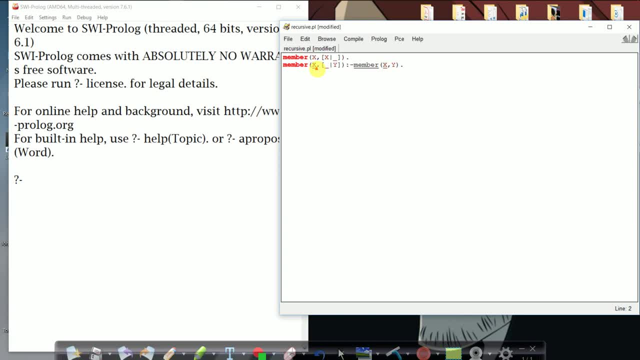 for the rest of the elements, if this x is present in head, then the first line will return as true. if it is not present in head, then it must be present in tail, which is y, and so here we will make the function call on the tail x and the tail. okay, and our tail. 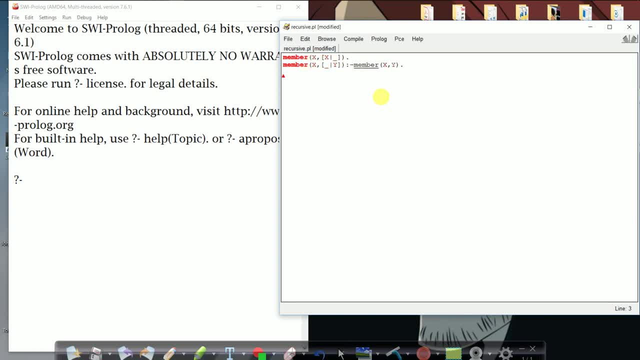 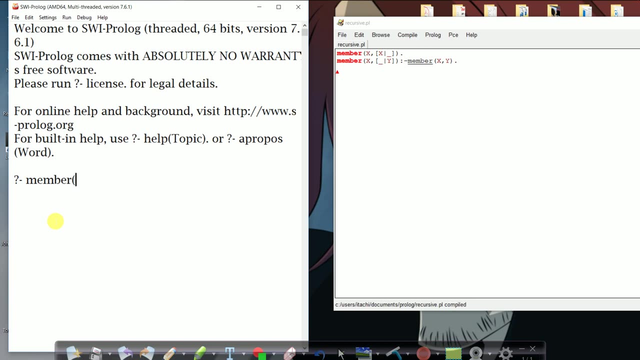 will be the entire list in the next function call. okay, so let us just save it and compile it. so i have compiled it and now we can run the code here we can write member and then give the access value as harry. okay, and now we can declare our list: adam comma carry, carry comma, harry comma john. so this is our entire.